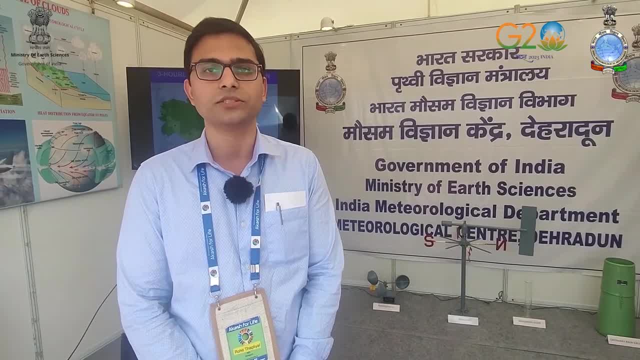 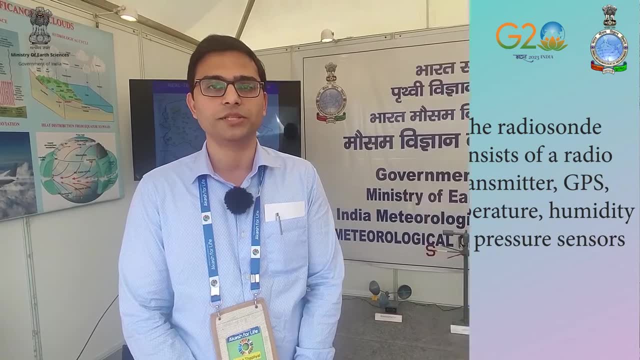 is attached, which is called a radiosonde. radio wind instrument is attached with it. This instrument has temperature sensor, humidity sensor and pressure sensor. Besides that, it has GPS chip, so its drag, from its drag we can track the wind speed and wind direction. 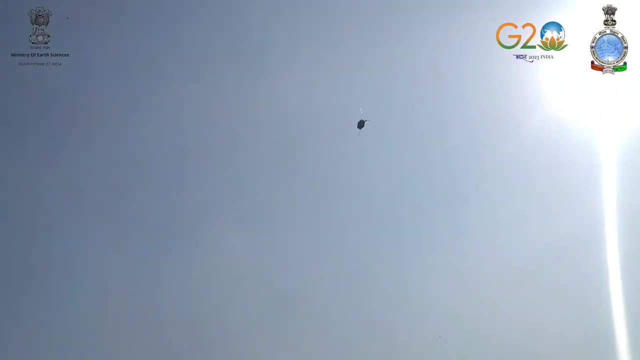 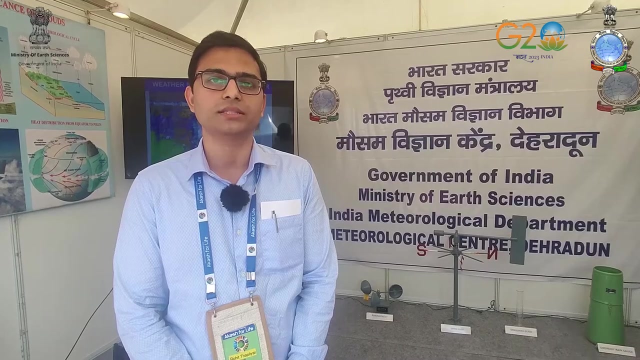 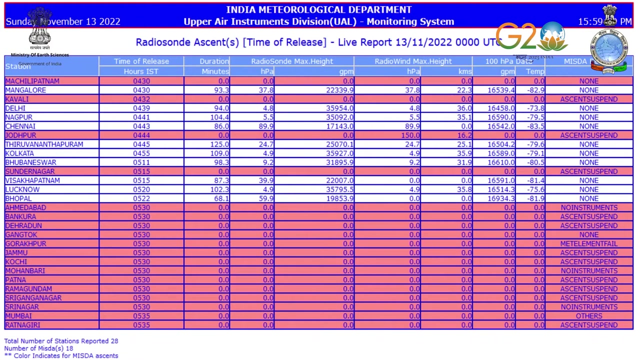 as well. So when the balloon is filled and the device is attached, it is released, So it goes up and it provides continuous weather information at every level. All these meteorological parameters like temperature, wind speed, wind direction, relative humidity, pressure, all 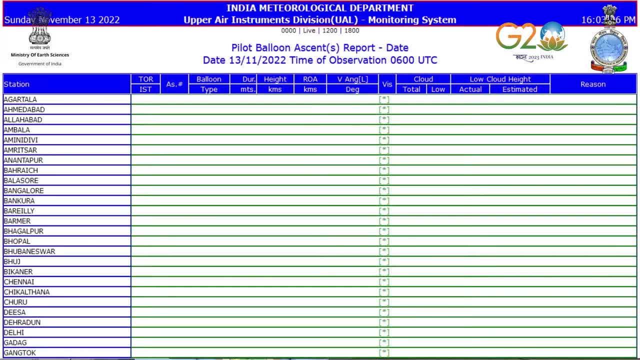 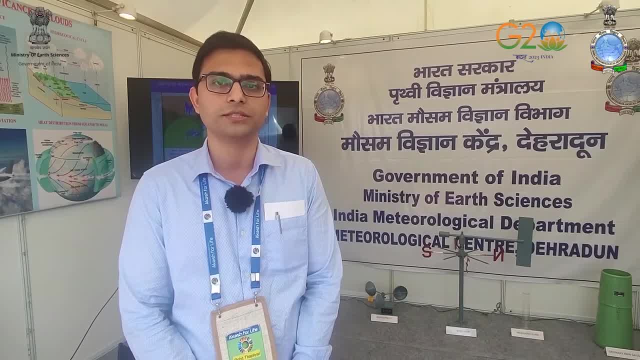 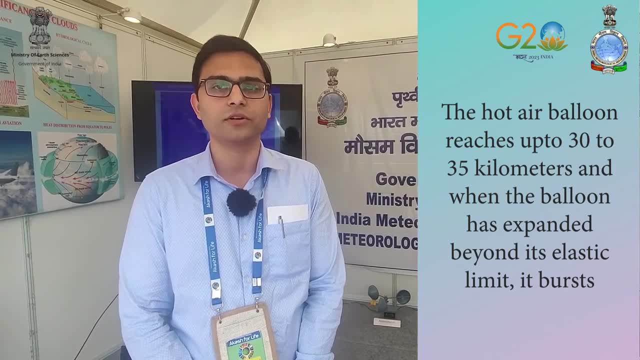 these parameters are received at the ground station. It continuously transmits and the observations are received at an interval of one second. So this balloon can reach up to 30-35 kilometers. After reaching 30-35 kilometers, the balloon bursts and the balloon along with the device. 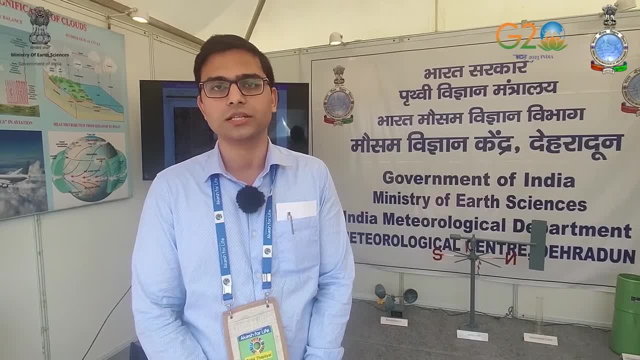 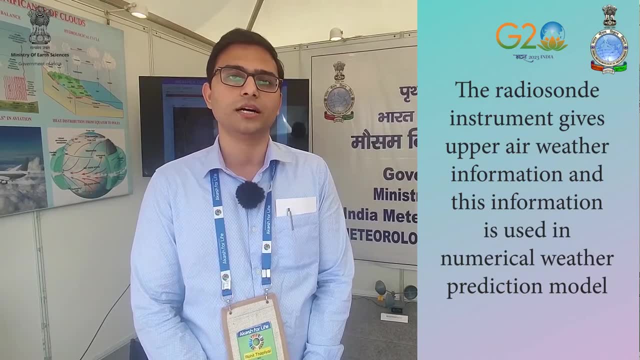 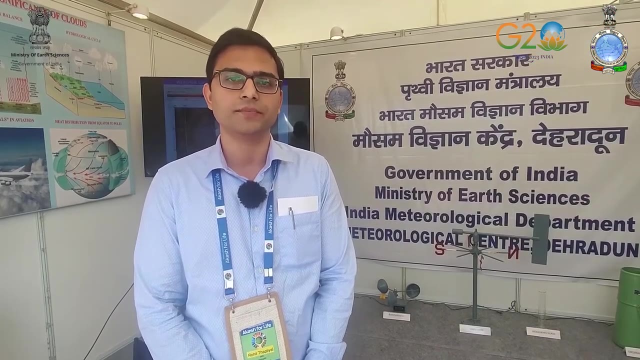 falls down. So it is a single use. currently it is a single use instrument, So it basically gives upper air weather information and this information is then used in a numerical weather prediction model as an initial condition. So there are many radiosonde, radio wind stations. 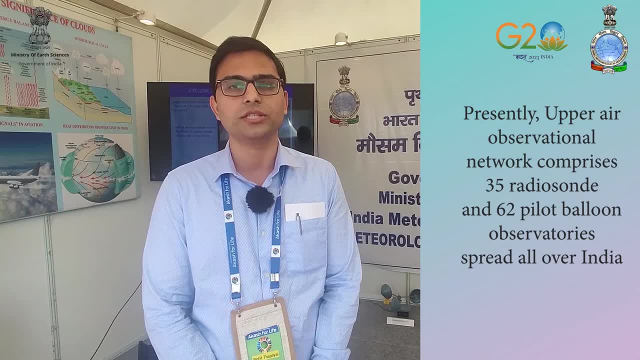 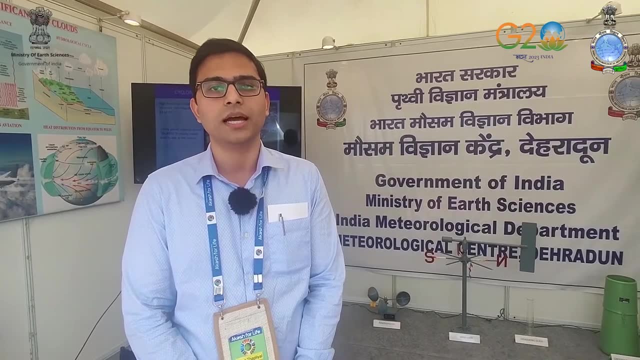 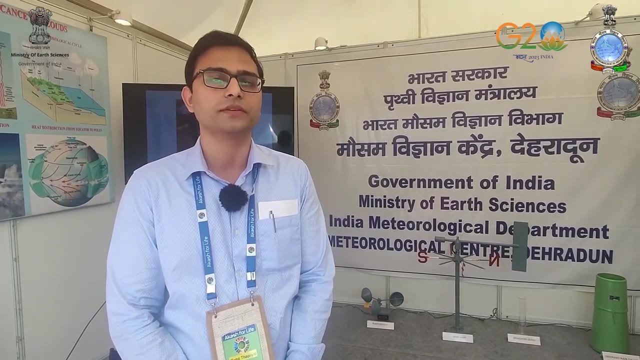 in India. These radiosonde radio wind stations are there in India which are taking these RSRW observations at synoptic hours, 0 UTC and 12 UTC hour. We have surface observation network, very good surface observation network, So we can easily get surface information. all these 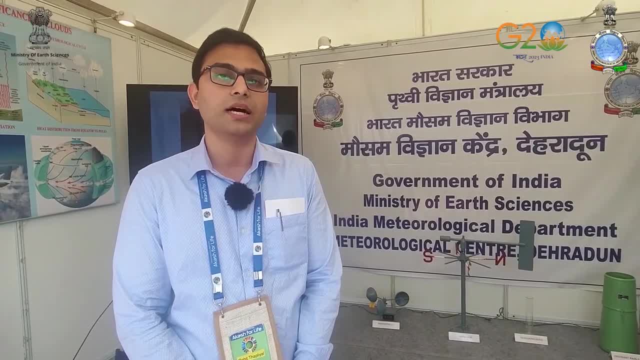 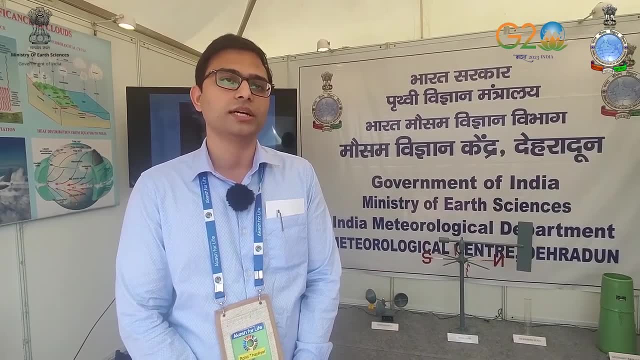 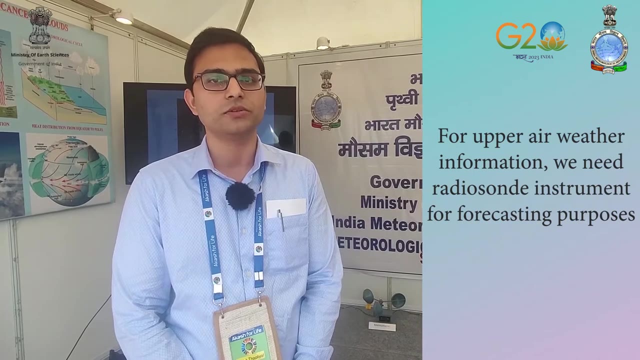 meteorological parameters at the surface, But upper air information is also important. So all the weather that happens, that happens in the troposphere. So for getting this upper air observations we need radiosonde devices. We also have pilot balloon observations, which only provides wind speed and wind direction data, But with the help of radiosonde radio. 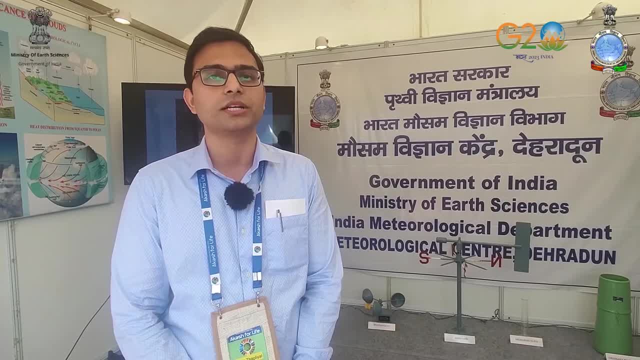 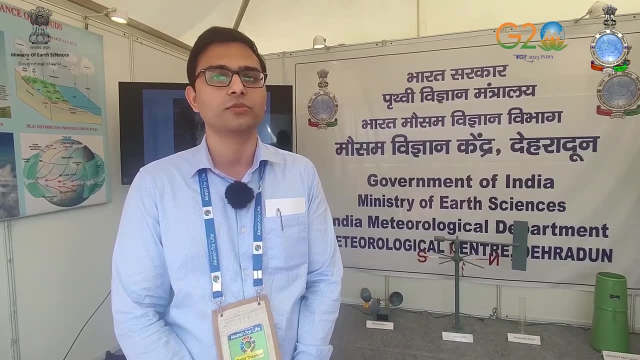 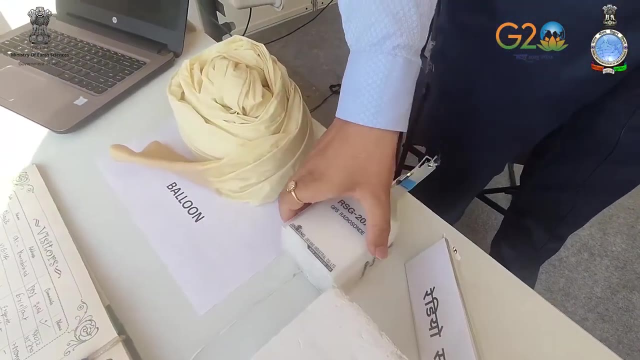 wind device. we can get additional data as well- temperature and humidity data- So it is important as an initial condition to be digested in the numerical weather prediction models for forecasting purposes. So this is the radiosonde radio wind instrument. So this instrument has radio wind instruments.